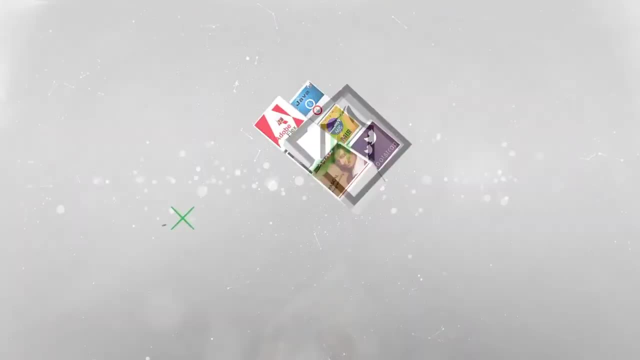 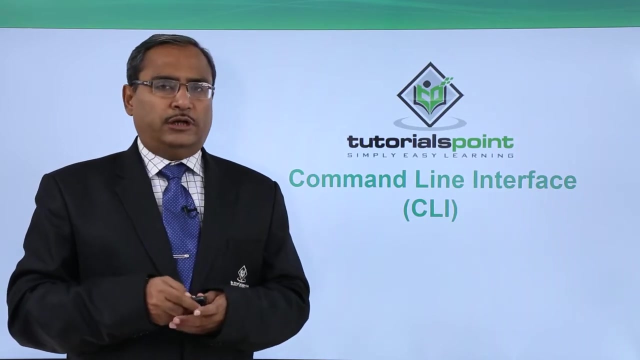 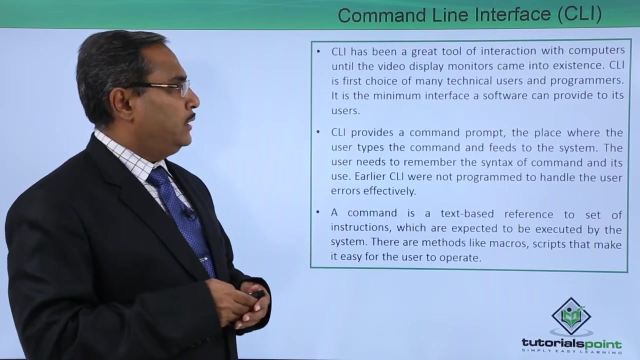 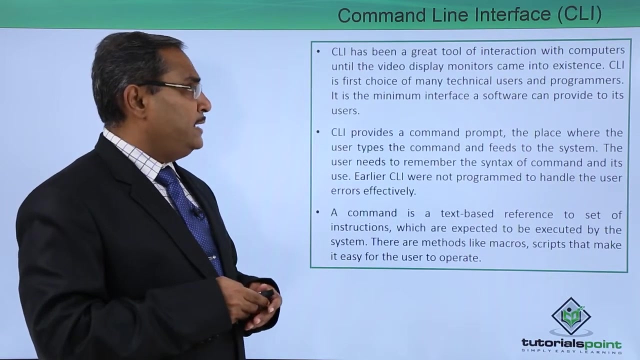 We are going to discuss command line interface. In short it will be called as CLI. So CLI has been a great tool for interaction with computers until the video display monitors came into existence. So CLI is the first choice of many technical users and respective. 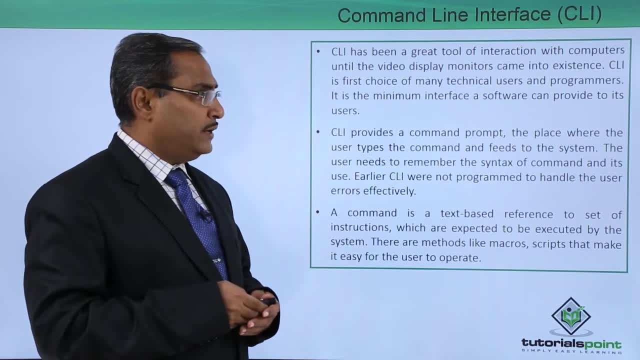 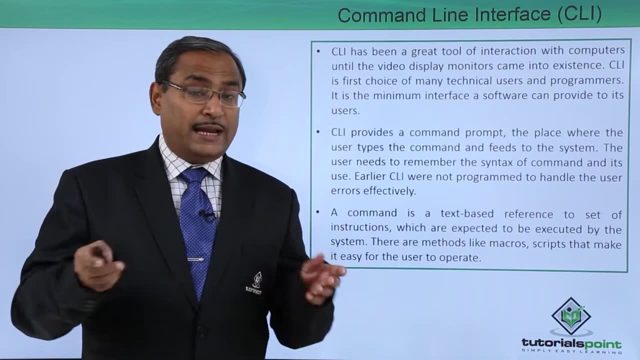 programmers, And it is the minimum interface a software can provide to its user, So those who are having the experience to work with the console, So they are actually using this CLI. So there is a command line interface where the commands will be issued and the 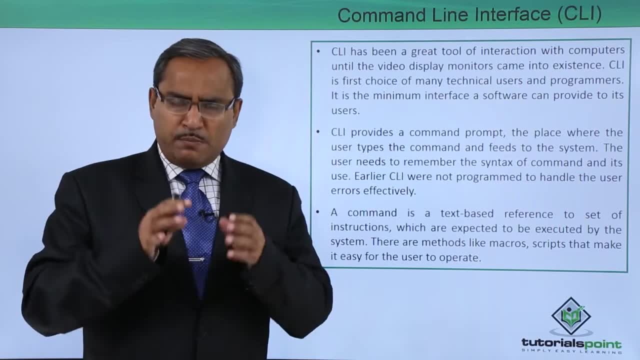 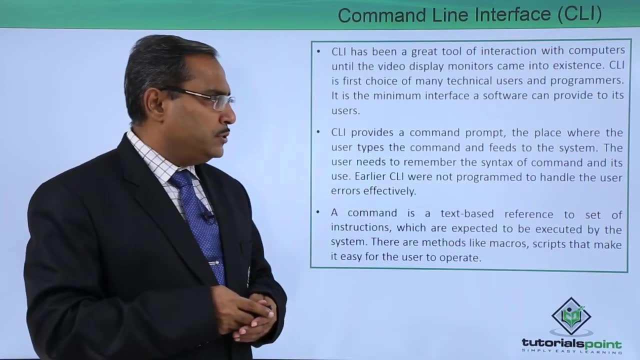 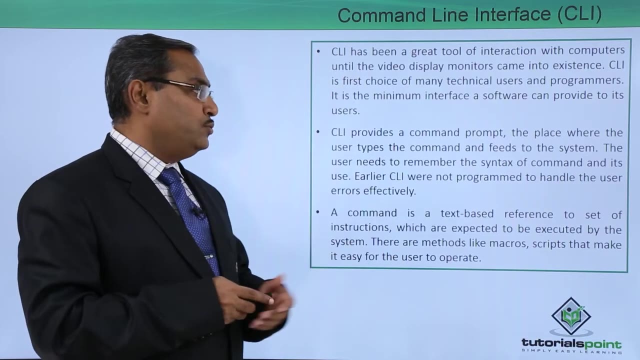 where the command will be issued and respective outputs will be obtained. So this is the minimum interface a software can provide to one user. So CLI provides a command prompt, the place where that user types the command And feeds to the system. The user needs to remember the syntax of the command and its 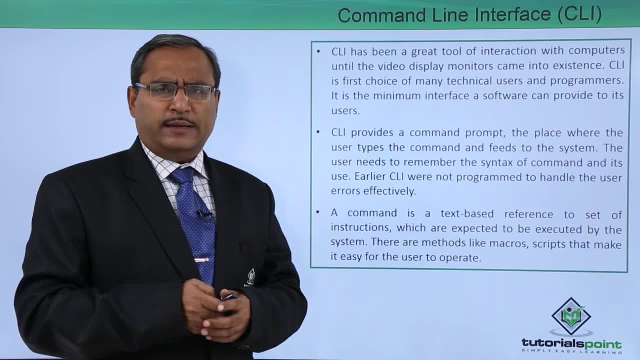 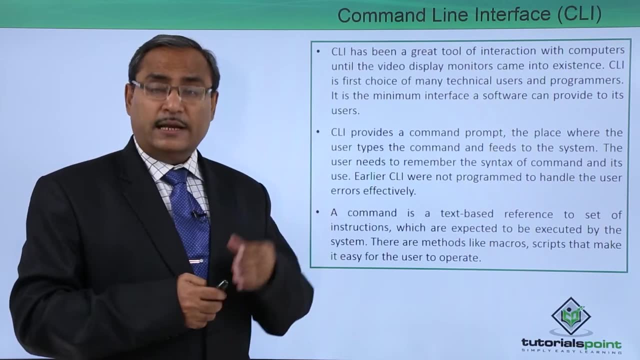 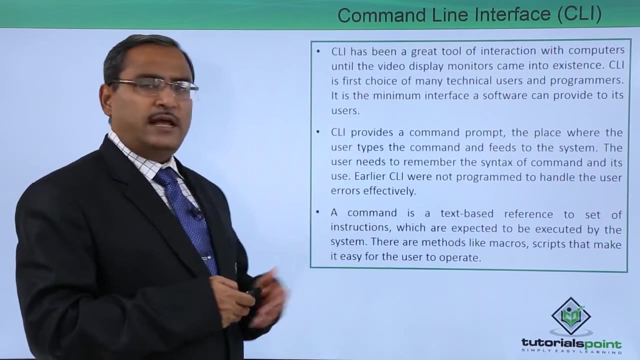 respective use. So depending upon the operating system, we know that there are different type of commands are there and each and every command has got different syntax depending upon the platform. So earlier CLI were not programmed to handle the user errors effectively. So 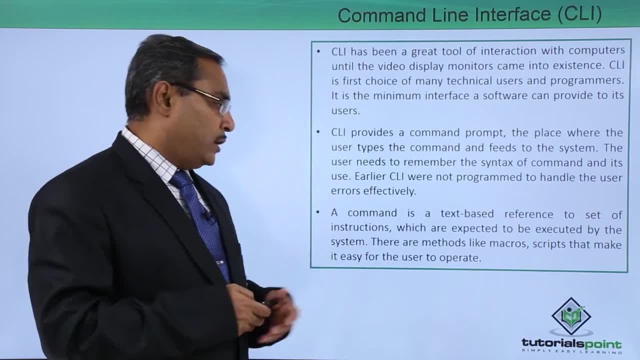 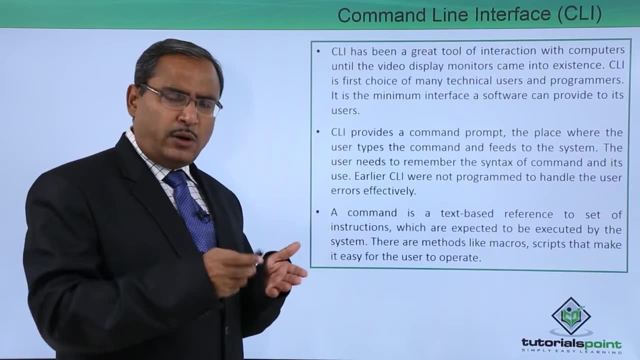 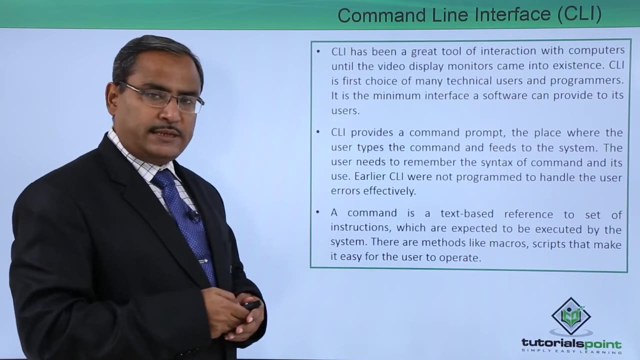 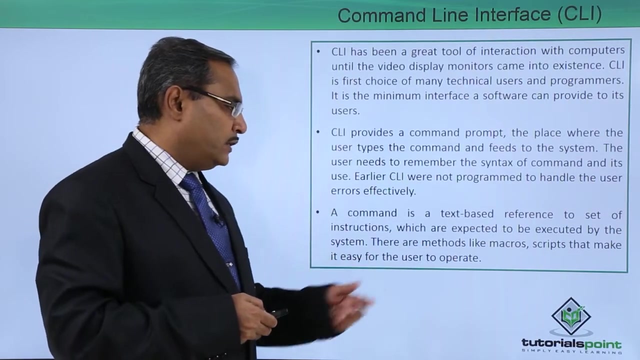 now let us go for the next point on this CLI. The command is a text based reference to set of instructions. So what is the command? Command is nothing but a text based instruction which are expected to be executed by the system, And there are methods like macros, scripts, that make it easy for the user to operate. 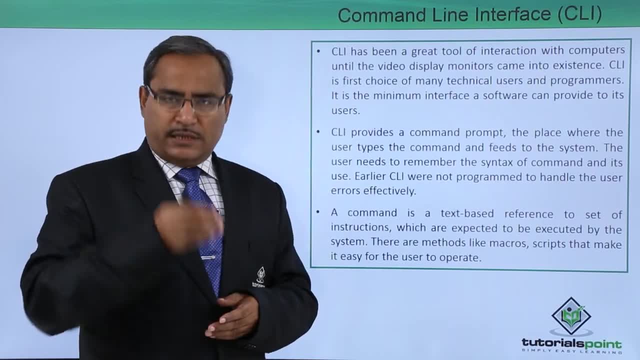 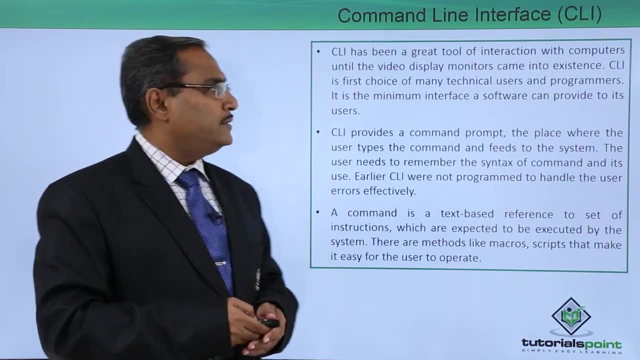 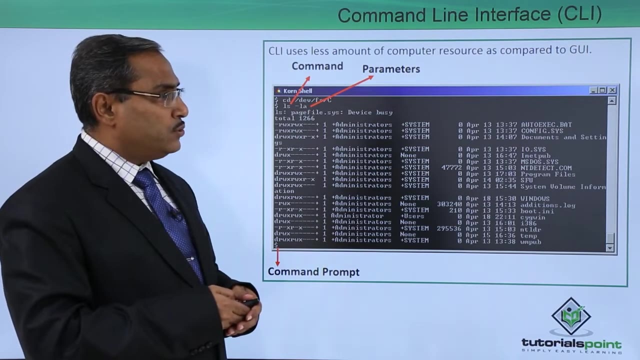 In a script we can write a set of instructions, set of such commands and instructions, And if we execute the script, then all those commands will get executed one after another. So here we are having. the CLI uses less amount of computed resource as compared to GUI, So 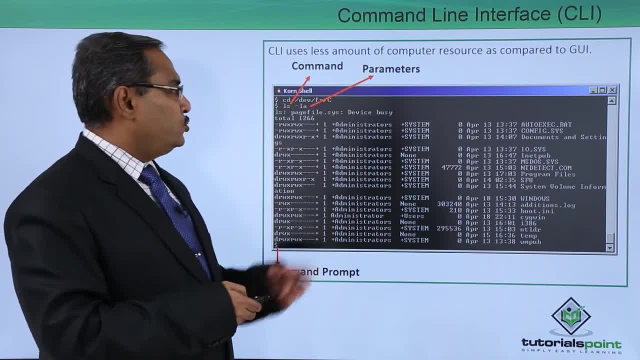 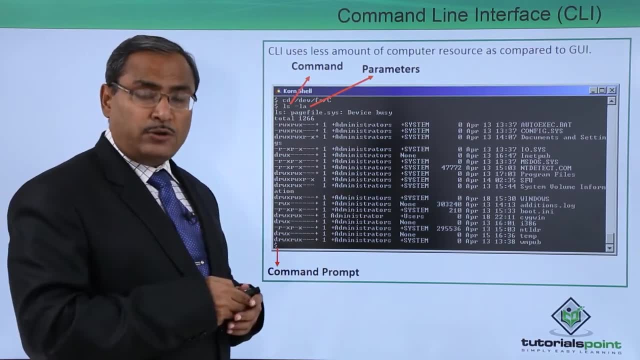 here we are having one Unix based CLI, So here we are having this prompt. This prompt is being denoted by dollar in case of, in case of Unix environment, Dollar indicates that you have logged as an ordinary user And if you have this hash symbol as an ordinary user, then you have this hash symbol as an. 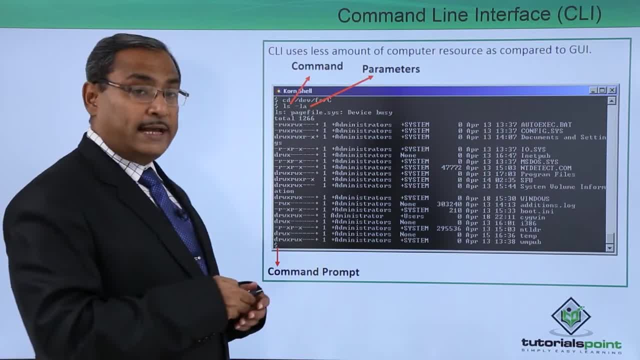 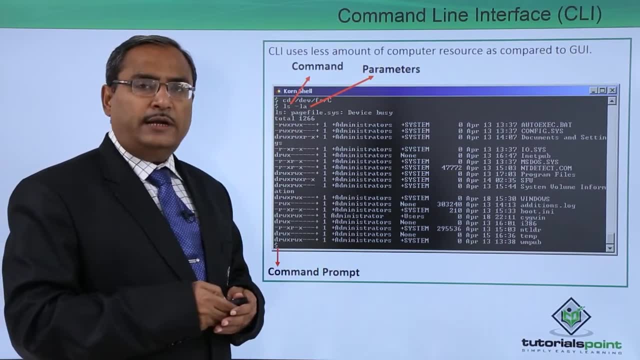 example, as a prompt. that means you have logged as a super user or as an administrator, So this is a command prompt. Here the command has been issued as LS. In case of Unix or Linux, LS stands for list, So this particular command has been issued, So this is a command. 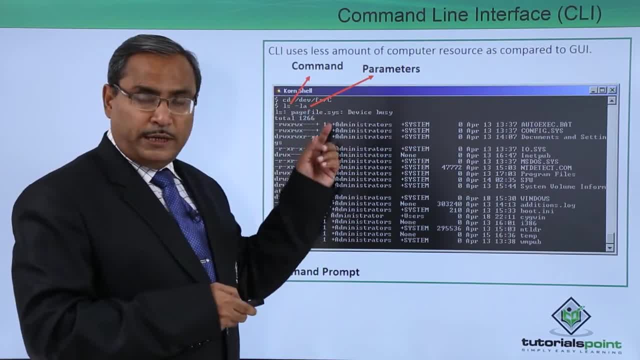 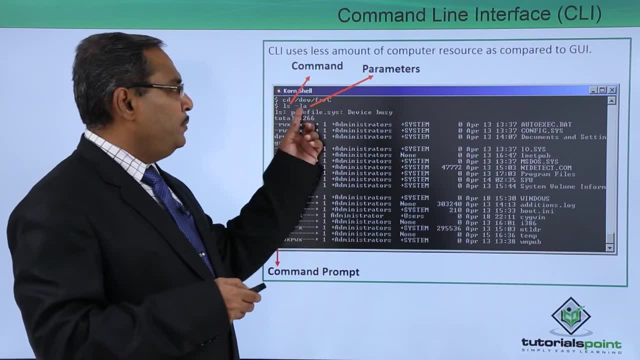 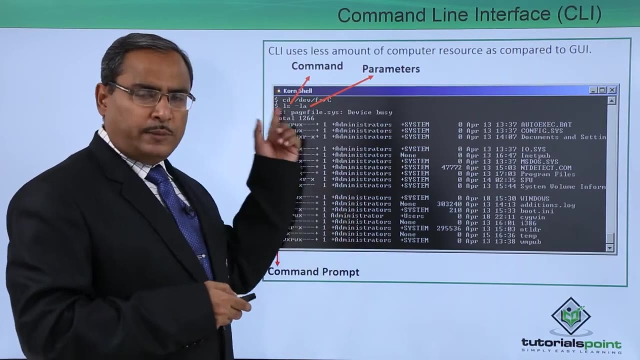 minus LA. So now all files are going to be displayed here, all the files, including the hidden one also, And L will be denoting the long list format, So they will be known as a parameters. with this LS command And this is a, respective outputs are coming. You see, everything is coming, Whatever the 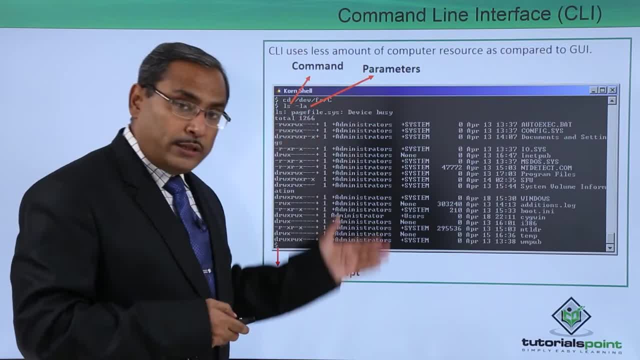 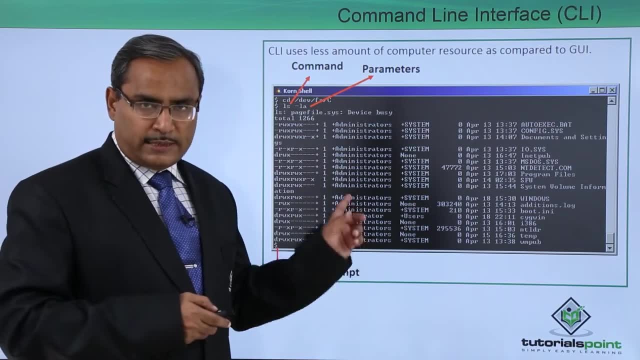 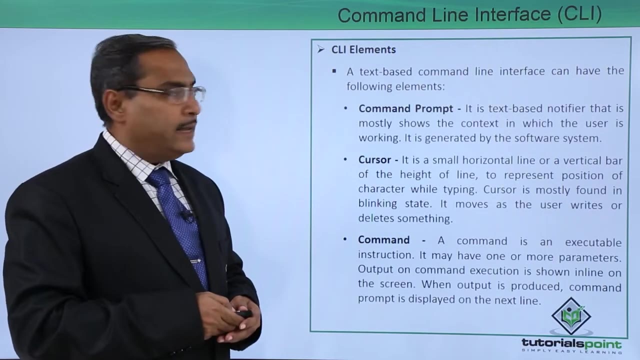 commands were executing. you are executing the command in the same screen where the outputs are coming, And here these outputs are having multiple different columns. So that is one console. as an example, We have put this one on our screen. Now let us consider the CLI elements. A text based command line interface can have the 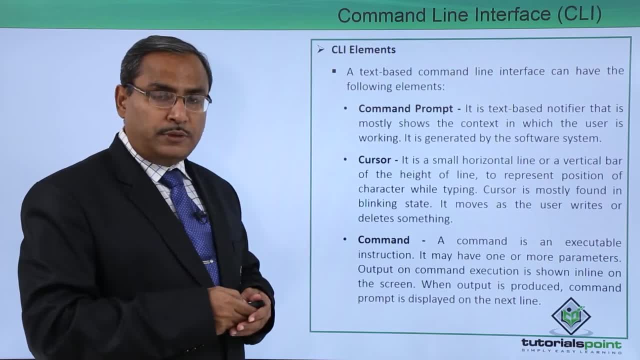 following elements. So what are they? We are having the command prompt. I discussed that one earlier. in case of Unix, If you log as a ordinary user, the command prompt will be your dollar. If you are the administrator or the super user, then your command prompt. 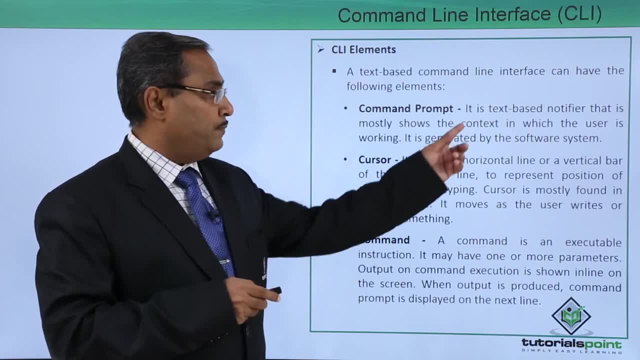 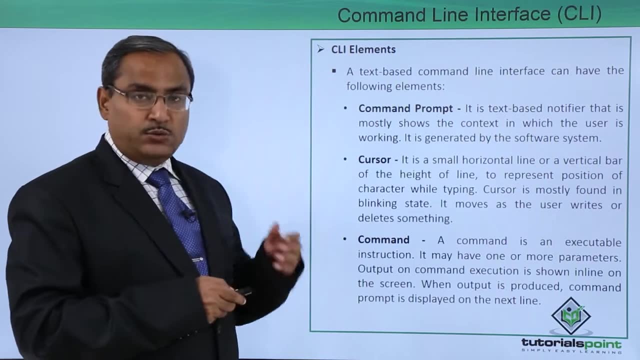 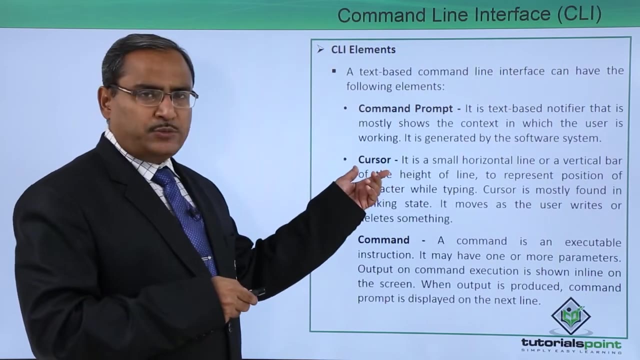 will be the hash symbol. There is a default one. You can change that one also. So it is a text based notifier that is mostly shows the context in which the user is working, And it is generated by the system software. There is a software system, So now next one. 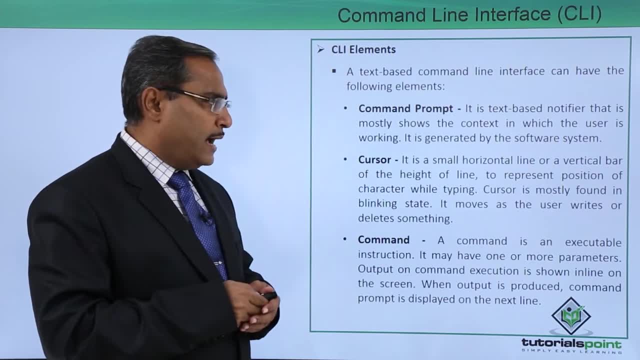 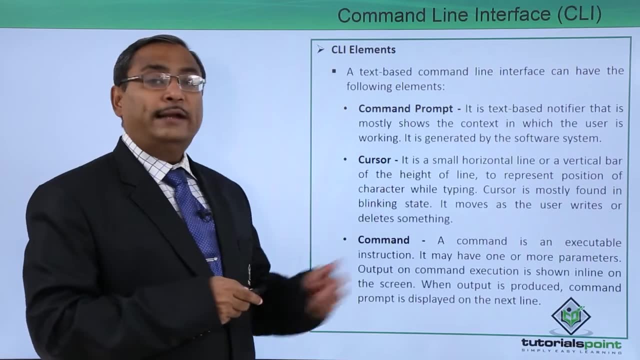 is the cursor. So this is a small horizontal cursor. So this is a small horizontal cursor. It is used to capture the position of the user. There is a vertical line, or might be a vertical bar also, of the height of the line, to represent the position of the character. 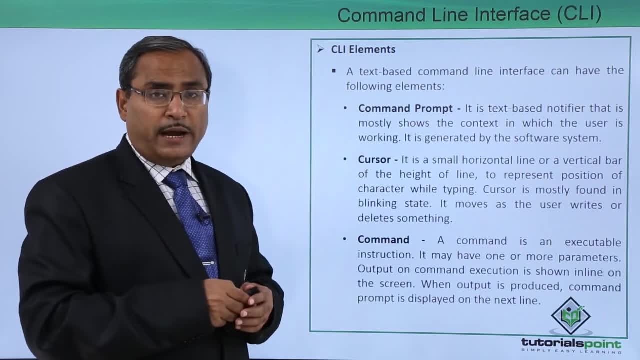 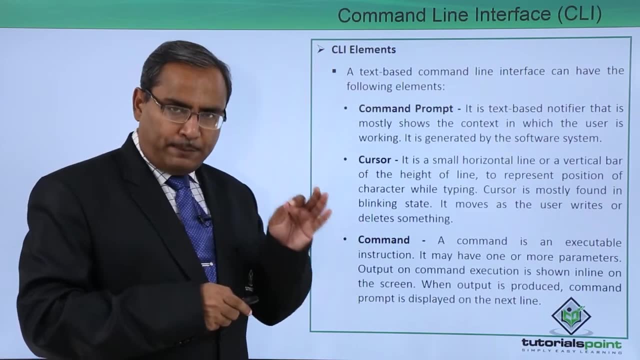 while tapping. So if we type the character on the keyboard, so where this character will get displayed on the screen, that will be denoted by the position of the cursor. So cursor is mostly found in blinking state to get to grab the attention of the user and it moves. 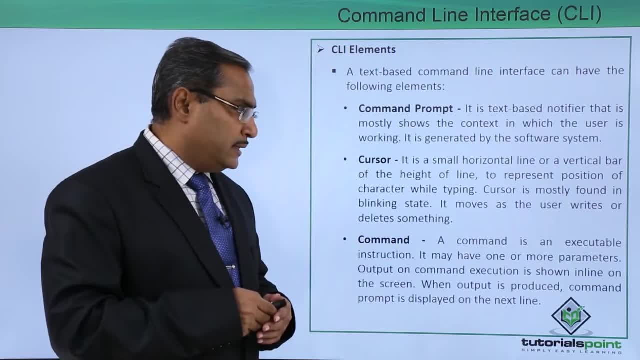 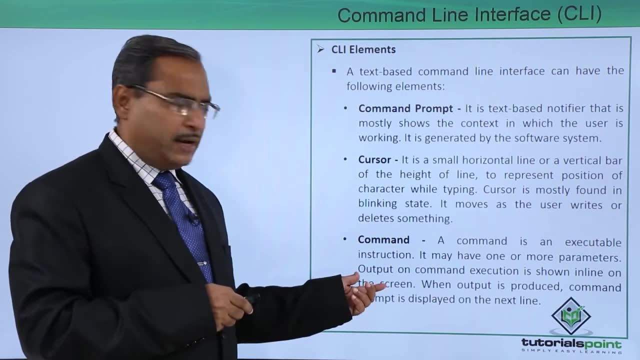 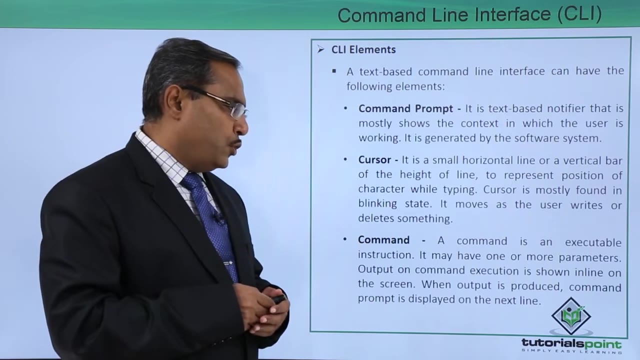 as the user writes or deletes something, nothing but an executable instruction. So it may have one or more parameters which you can pass with the commands and output on the command execution is shown in line on the screen. When output is produced, the command prompt is displayed on the next line. So